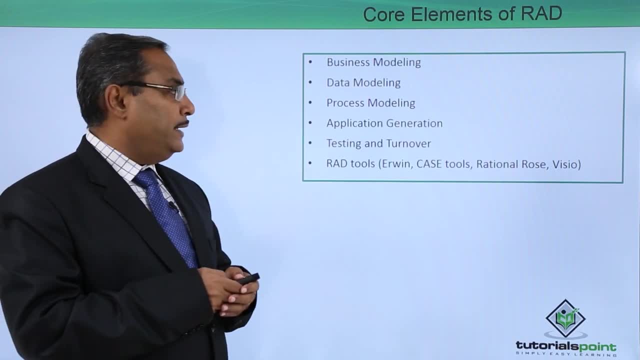 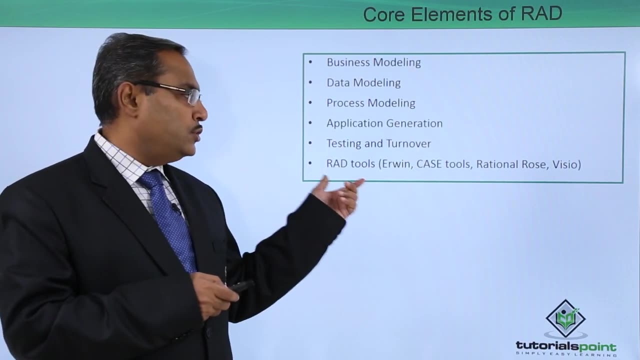 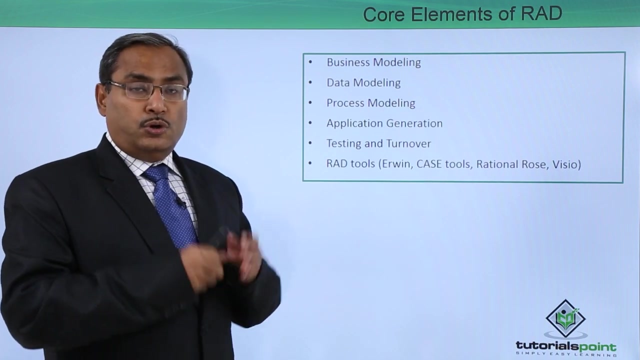 modeling, data modeling, process modeling and application generation, testing and turnover, and we are having multiple different RAD tools. So these are the set of RAD tools which we are using a nowadays. also, we are using this RAD tools. we are using Whenever we can develop a software depending upon, based on multiple different components. 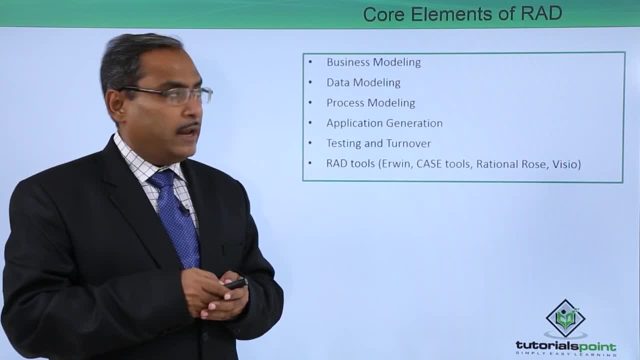 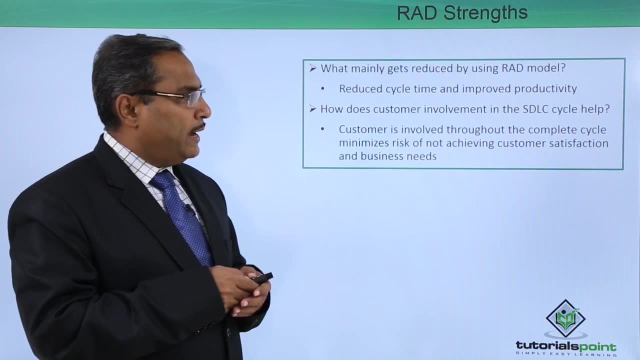 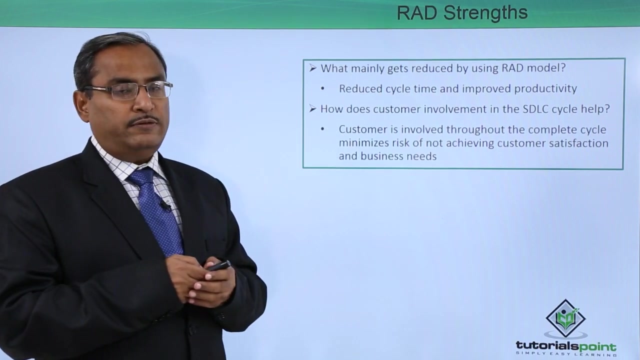 then only this RAD model can be applied. So let us go for the RAD strengths. So what mainly gets reduced by using the RAD model? This is, if this is a question, the answer is the reduced cycle time and improved productivity. So it will improve the productivity because 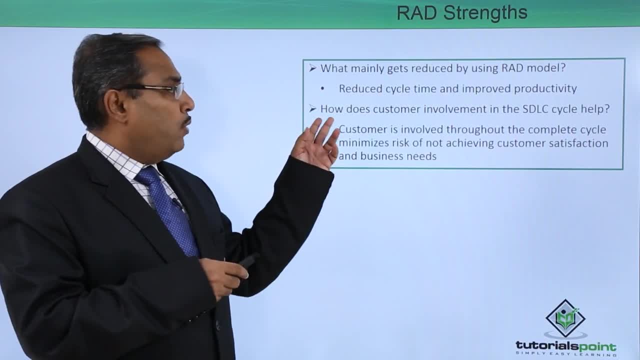 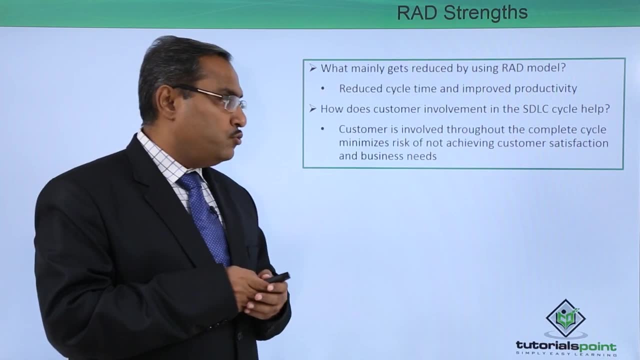 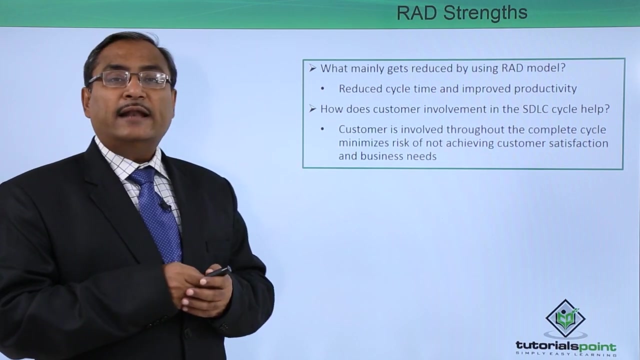 multiple teams can work on these components, And how does customer involvement in the SDLC cycle help? The customer is involved throughout the complete cycle, minimizing the risk of not achieving customer satisfaction and the business needs, So as customer is having a continuous participation in this development. 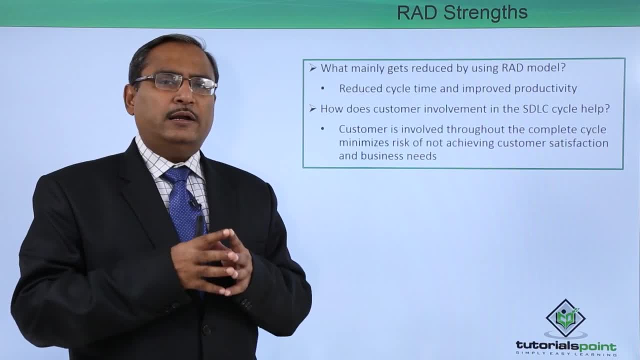 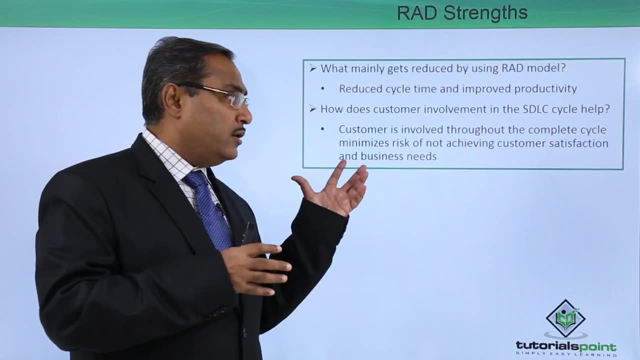 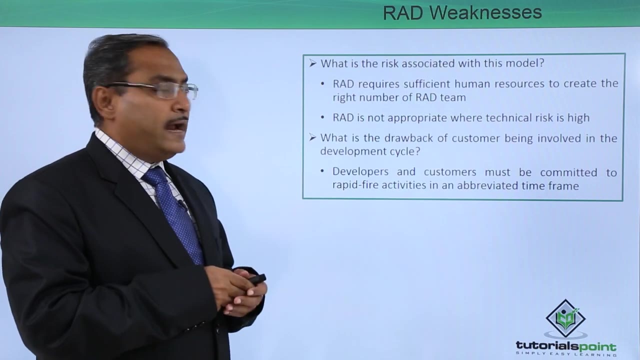 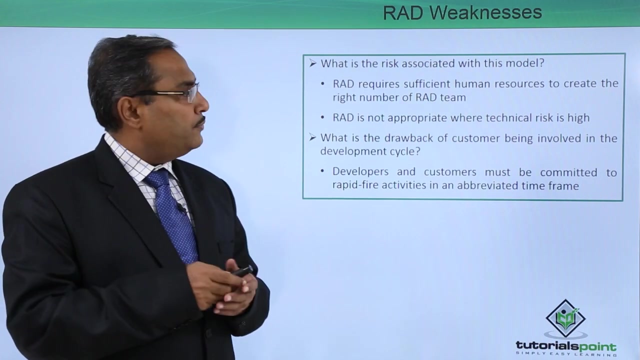 model. So the risk is very low that ultimately, the product which is going to get developed will be not in accordance with the customers requirements. Now let us go for the RAD weaknesses. What is the risk associated with this model? We know that risk means cost of failure, So RAD requires sufficient human resources to 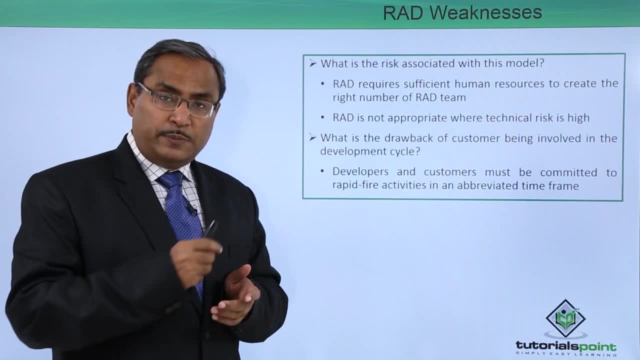 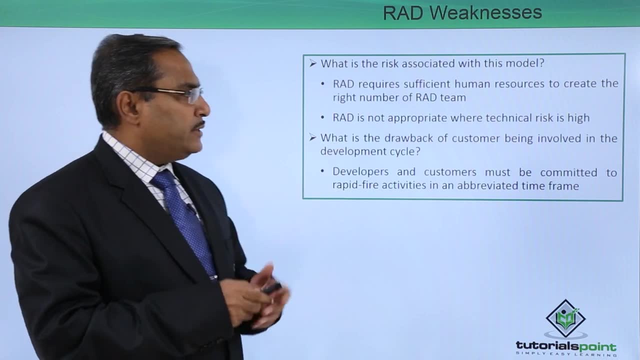 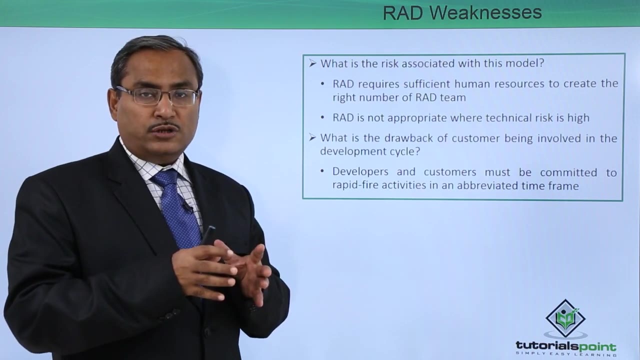 create the right number of RAD teams, as multiple teams will be working simultaneously in parallel, So huge manpower is required here. RAD is not appropriate where technical risk is high. If you do not not, if you are not confirm enough that this particular technology, this particular technique will be the fruitful, 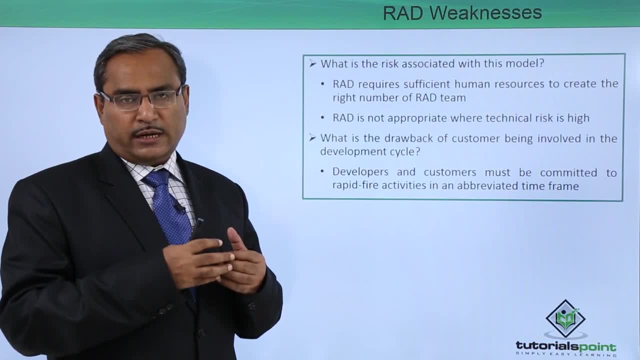 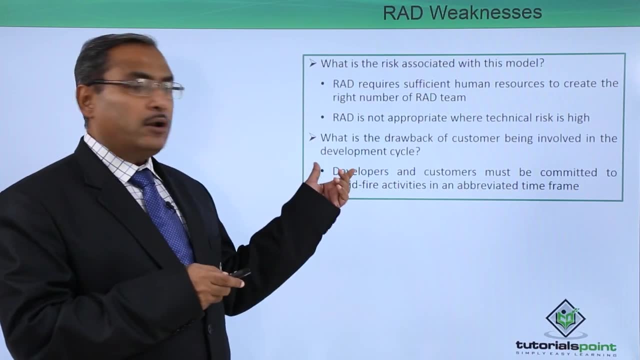 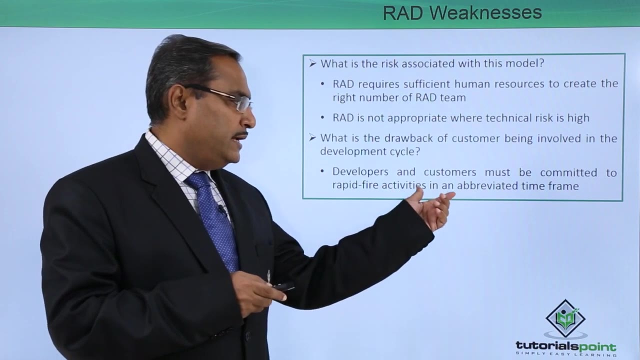 one where we are not having executed any kind of pilot project earlier. in those cases, this RAD is very much risky. What is the drawback of customer being involved in the development cycle? The answer is: developers and customers must be committed rapid fire activities in an abbreviated time frame in. 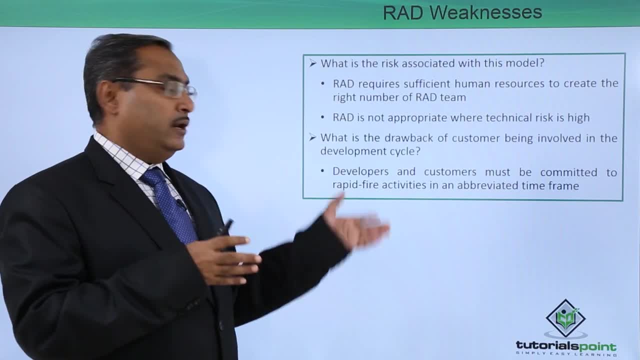 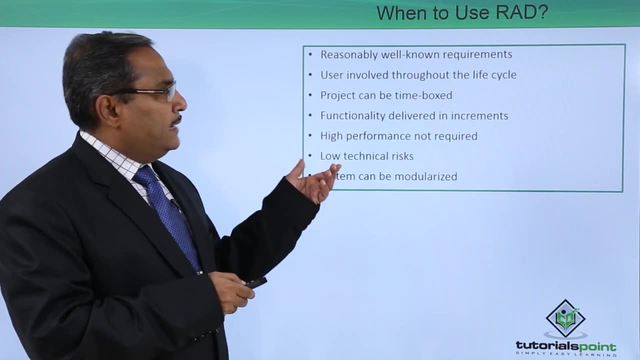 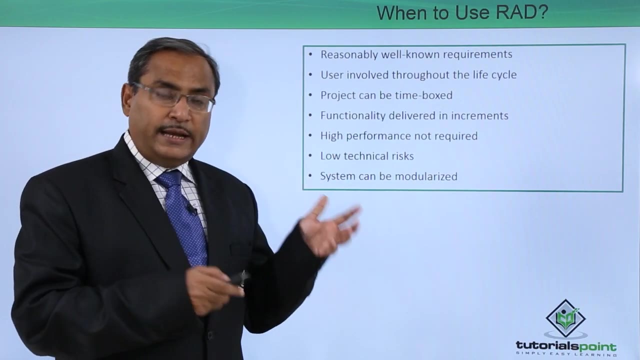 a certain time frame. in a very short time frame, this particular applications are to be developed. Now question is that when to use the RAD model? The answer is reasonably well known requirements: User involved throughout the life cycle. There, only this RAD model can. 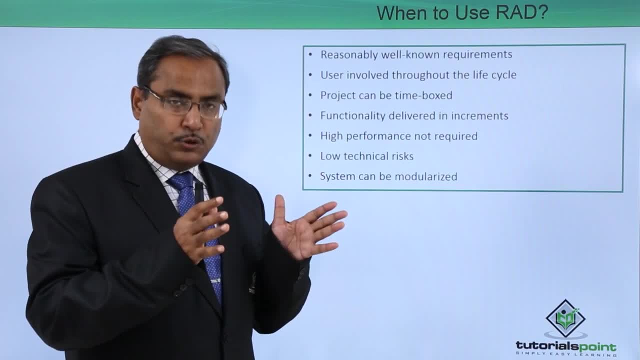 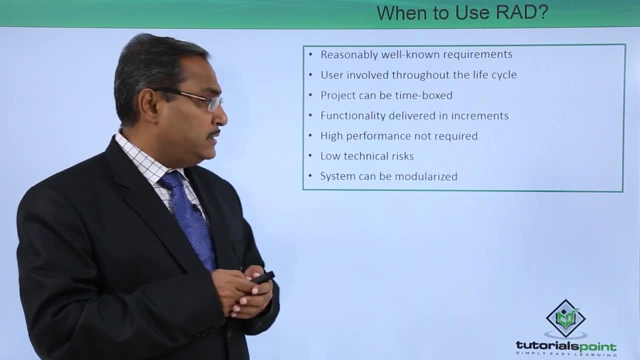 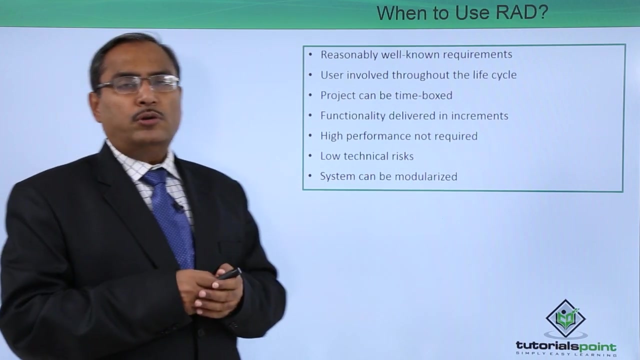 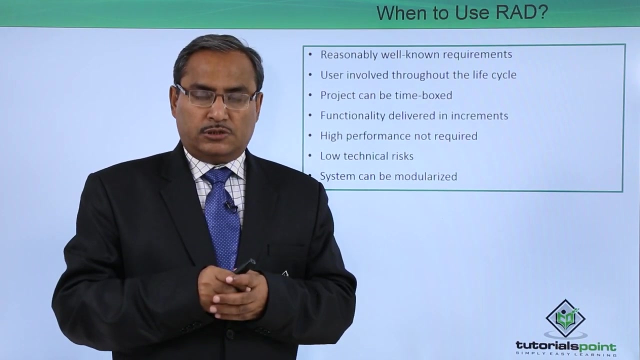 be implemented. Project can be time boxed- The project has to be executed within a very stipulated time frame and then functionality delivered in increments, high performance not required and low technical risks. and system can be Modularized and can be broken down into multiple, Non overlapping components. so I think you are getting this idea. What is the red model? 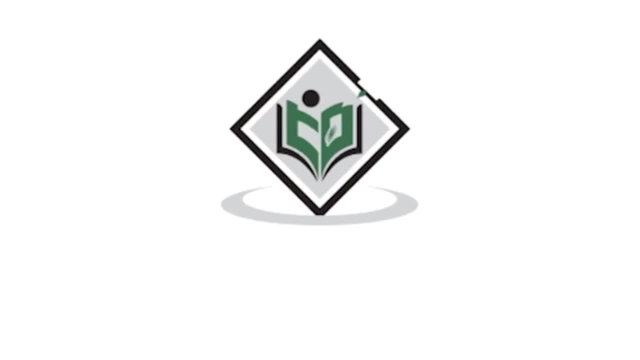 Thanks for watching this video tutorials: point calm, simply easy learning. 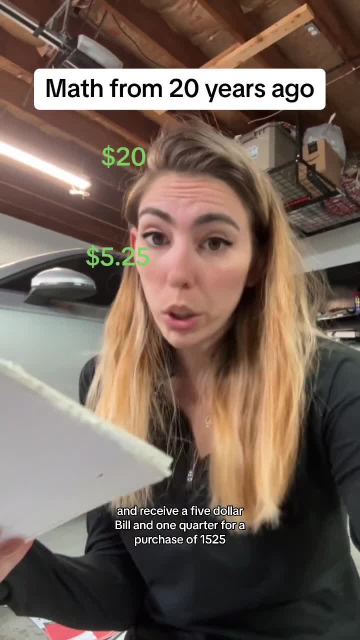 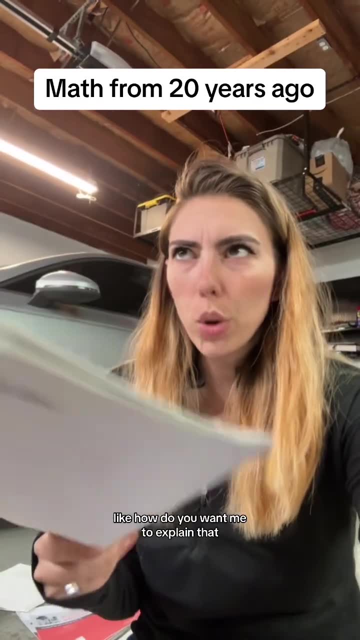 You give the clerk a $20 bill and receive a $5 bill and one quarter for a purchase of $15.25.. Was the correct change given to you? Explain, Explain what Like. how do you want me to explain that Like? you want me to do the math and then, or like, write a written description and explain. 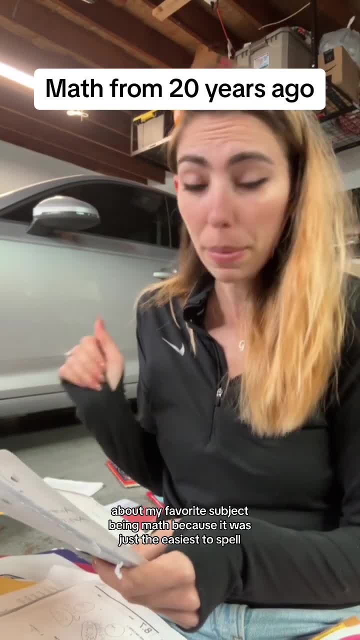 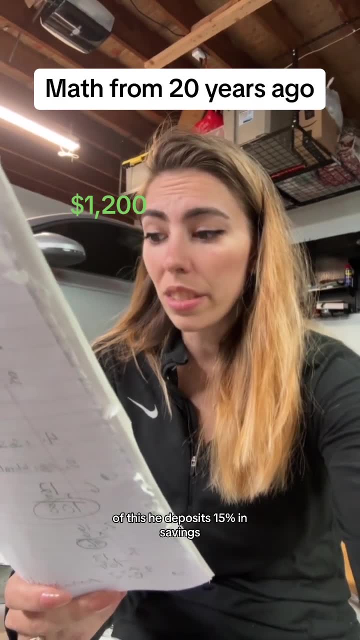 How would I? I'm beginning to think that I lied to my first grade teacher about my favorite subject being math, because it was just the easiest to spell. Jeffrey earns $1,200 per week In 2003. of this, he deposits 15% in savings. How much does Jeffrey put into savings each week? Honestly good. 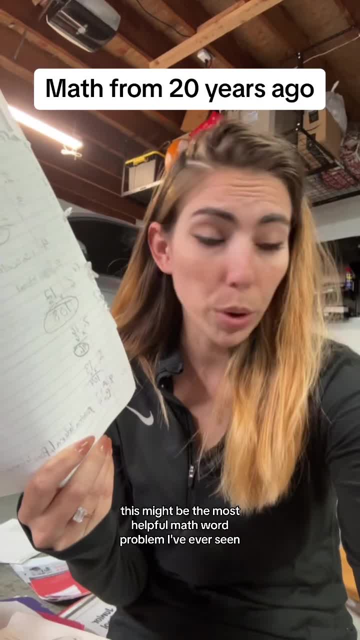 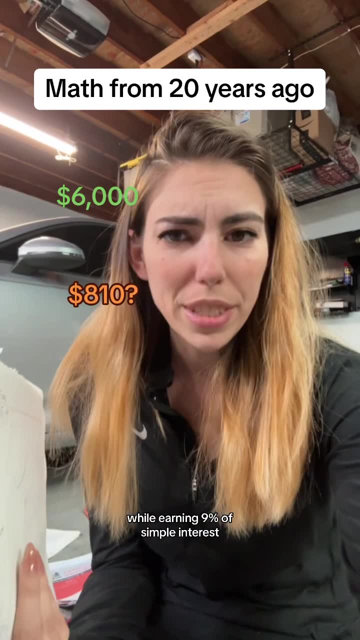 for you, Jeffrey, in 2003.. Second of all, this might be the most helpful math word problem I've ever seen. You deposit $6,000 in savings. Determine how long it would take to earn $810 while earning 9% of simple interest. But like, why in the second grade was I? Why not like high school? What Same. 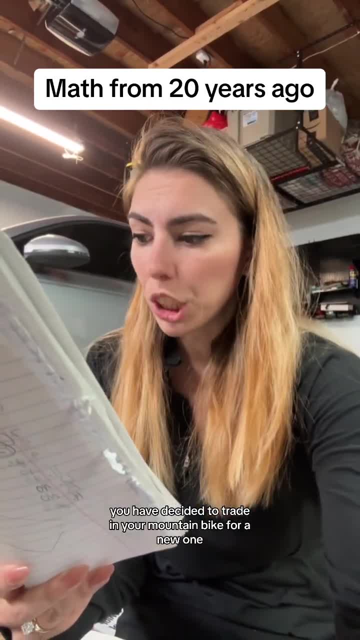 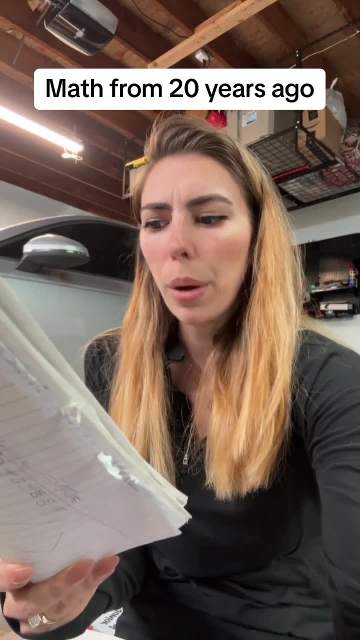 questions High school. You have decided to trade in your mountain bike for a new one. The bike shop stated they will give you 42% of the price of the old bike, or $226.. What was the price of your old bike? Again, second grade. 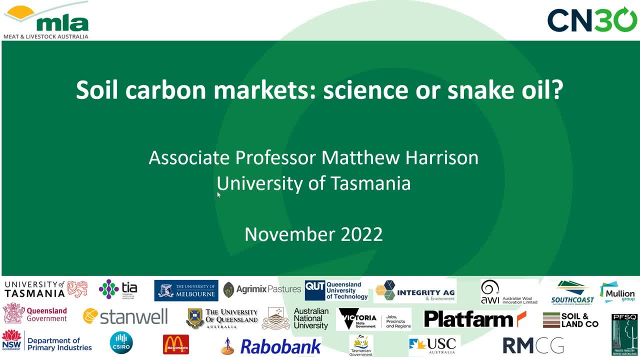 Hello, my name is Matthew Harrison. I'm a farming system scientist at the University of Tasmania in Australia. Today I'll be talking about soil carbon markets, whether it's science or snake oil. I recently did this presentation by invitation to a large international bank.